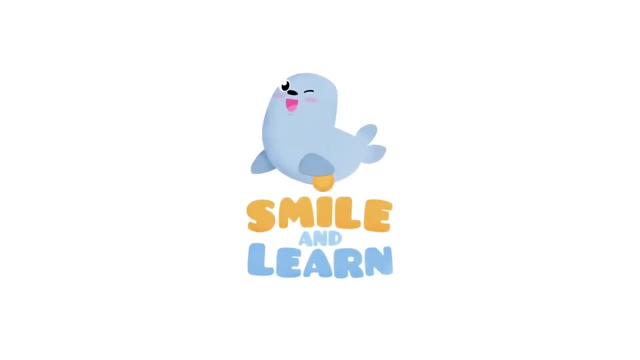 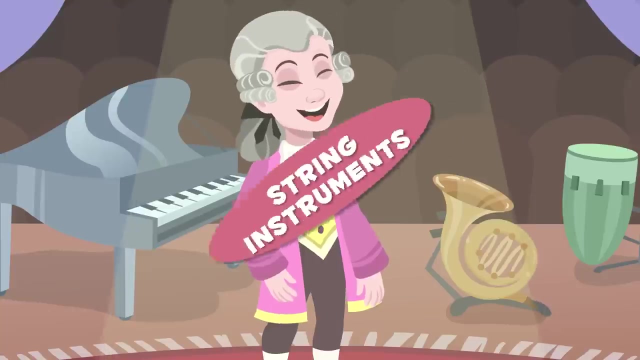 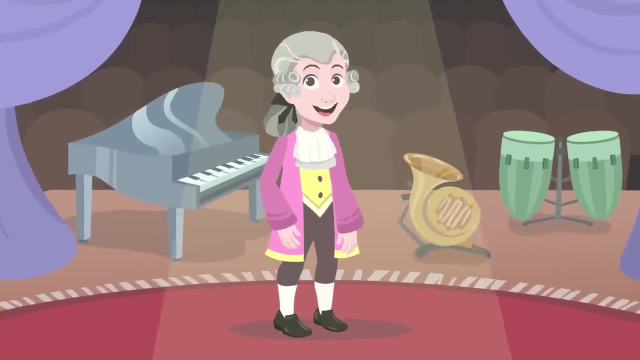 Hey friends, today I'm going to teach you about string instruments. Are you coming along? The instruments in this family have different strings. When they are played, we hear different music notes. Do you want to see some string instruments? Let's go for it. 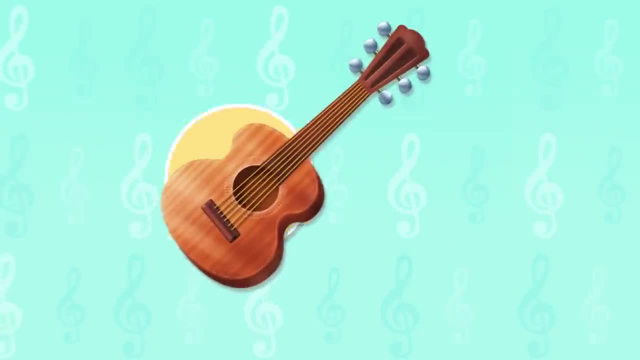 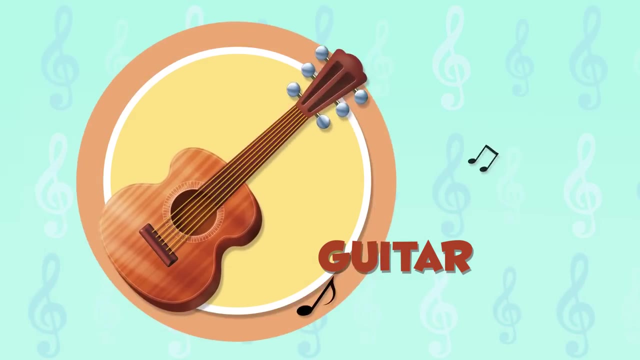 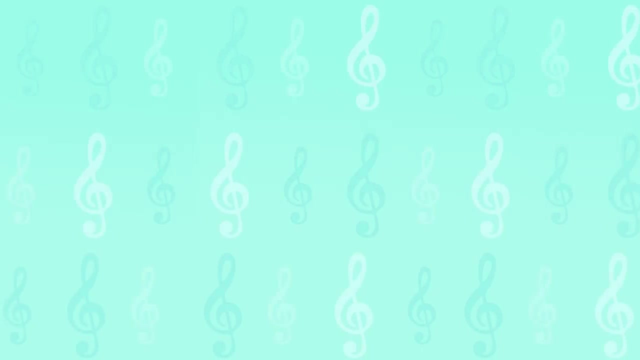 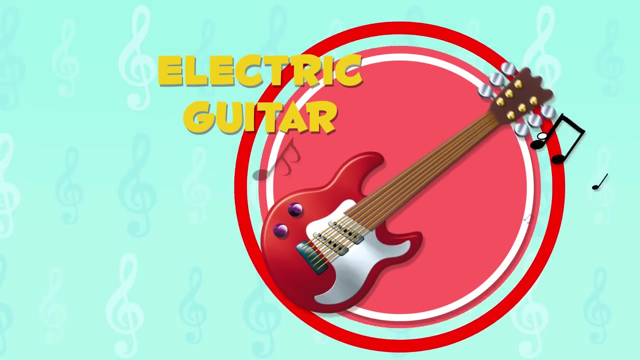 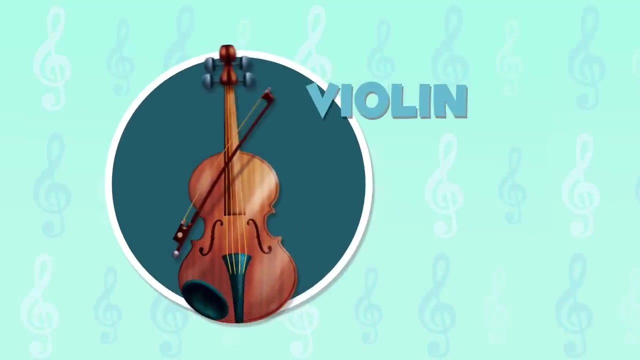 The guitar is a six-string instrument. It is used a lot in flamenco music. This is what it sounds like. The electric guitar is used a lot in rock music. Listen to its sound. Wow, I love how it sounds. The violin has four strings. The musician places it under his chin and it is played. 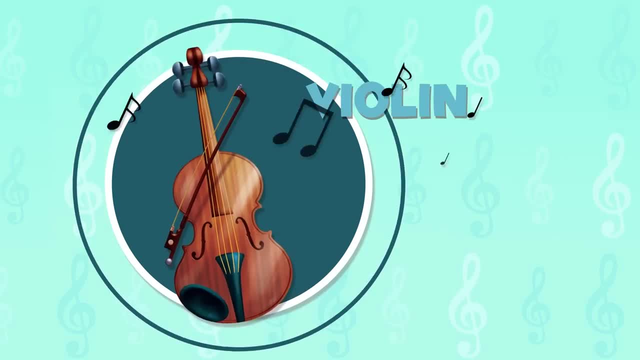 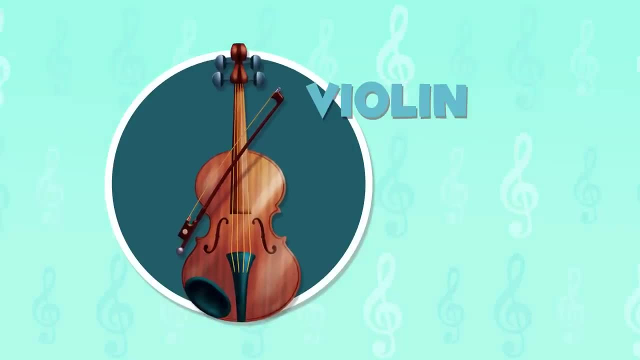 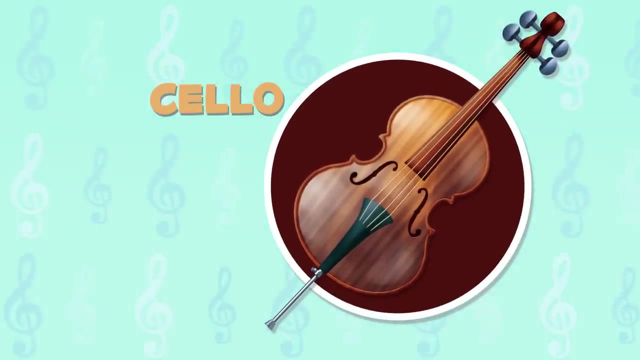 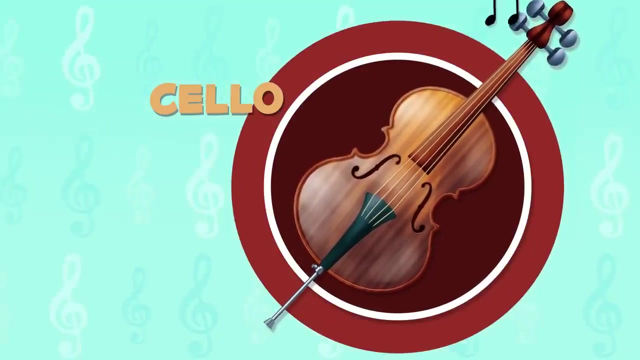 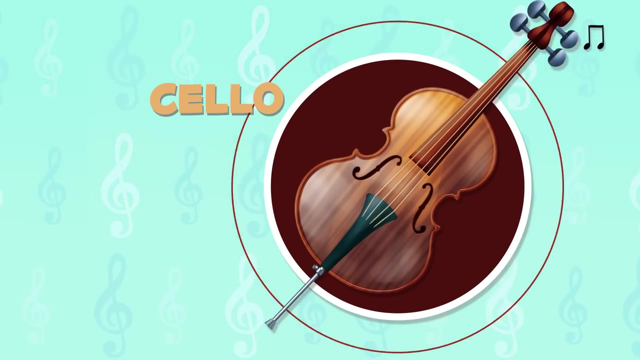 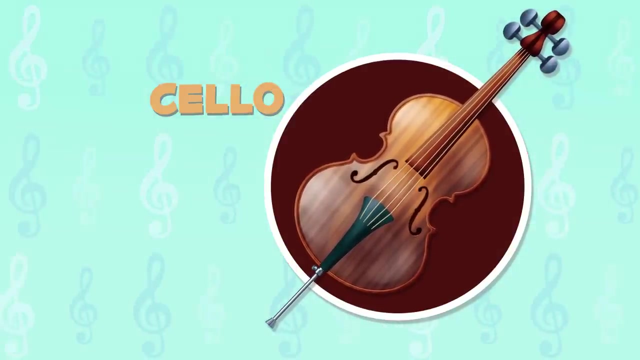 by strumming the strings with the bow. Have you heard how it sounds? It is really soft and nice. The cello is an instrument belonging to the violin family and it is also played with a bow. What a beautiful sound. The ukulele is a small guitar with four strings. 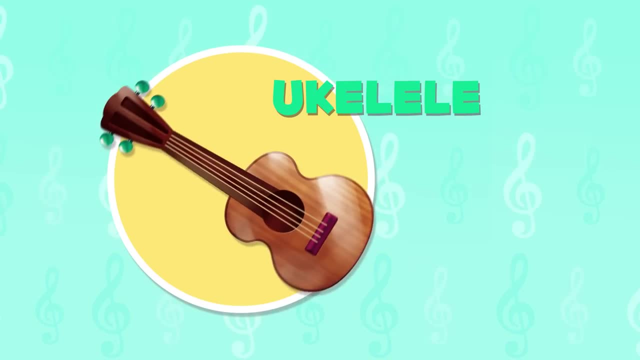 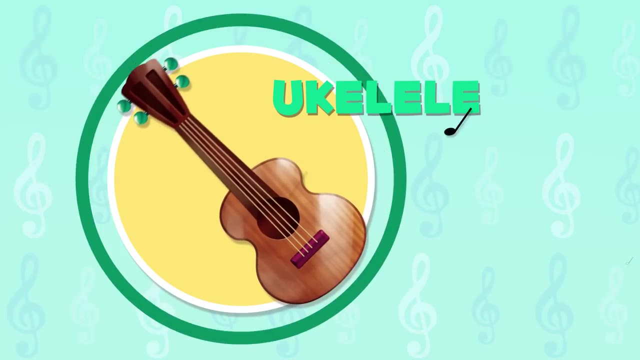 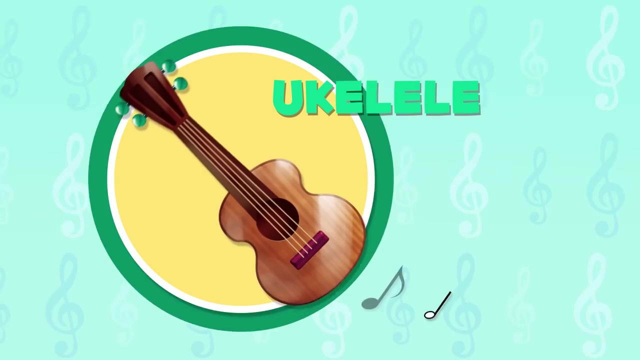 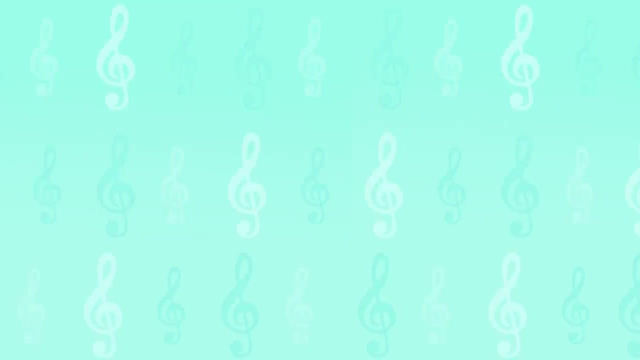 In Hawaii they play it with the hula band. Do you know what it sounds like? It sounds great. That harp has up to 39 strings and they produce sound when they are plucked by the musician's fingers: Silence. 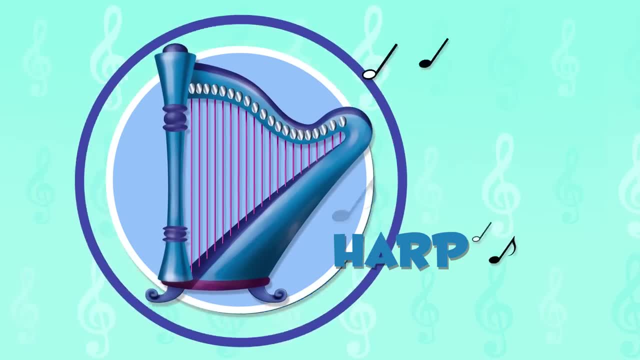 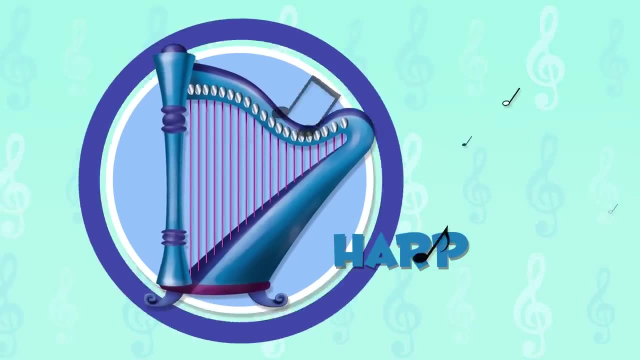 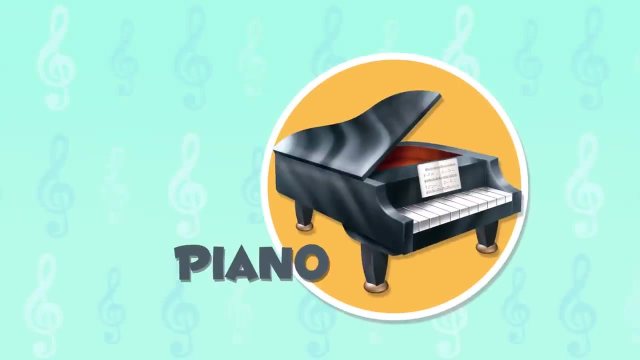 Shh. We are going to listen to how it sounds. The piano is the exception. Inside it has 230 strings that are hit by hammers under the keys. It is one of the most important instruments and is also considered a percussion instrument.